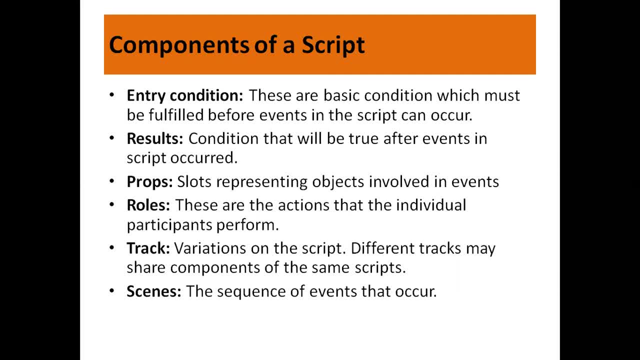 A simple example: if you want to catch a bus Now, what is the entry condition? you must be standing on the bus stop Now. results condition: that will be true after events in the script occur When the person could catch the bus. Props: The slots representing objects involved in the event. 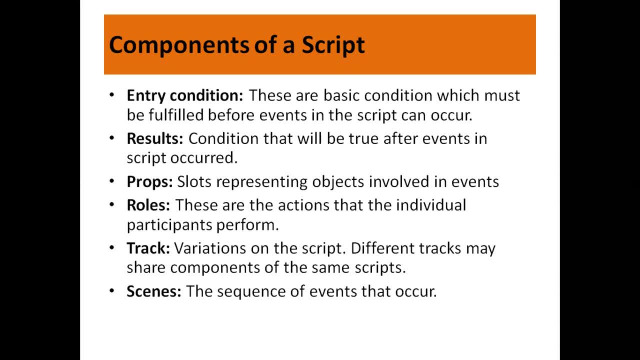